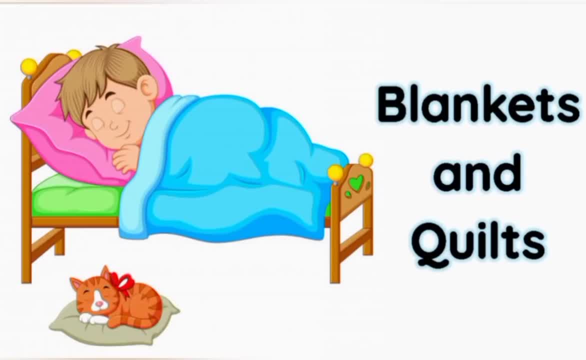 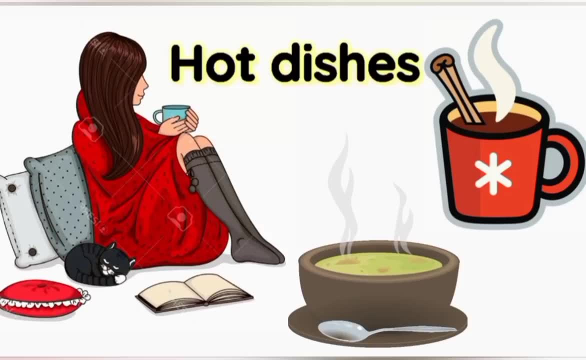 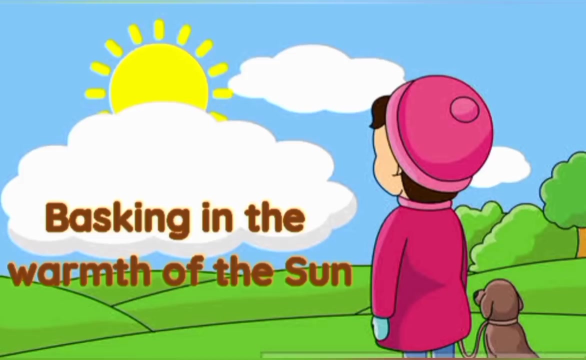 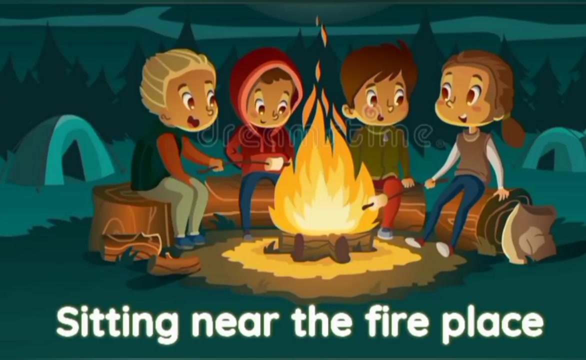 also use blankets and quilts In this season. people prefer to stay indoor and love hot beverages and relishing hot dishes wishes. In the daytime we like to bask in warm sunshine, and at night we often see people sitting near the fireplace to keep themselves warm. During this time, the days are shorter. 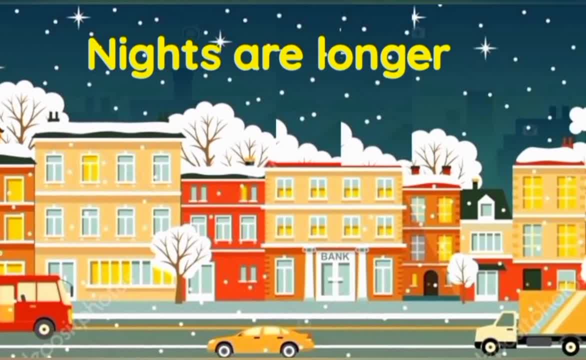 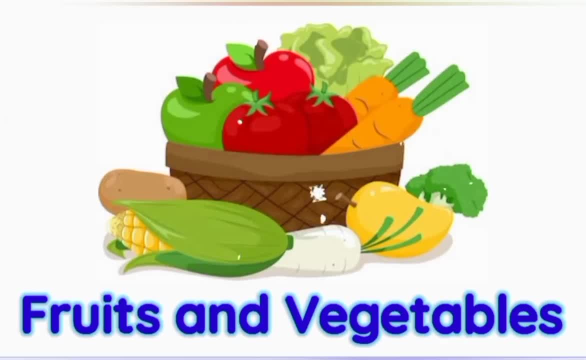 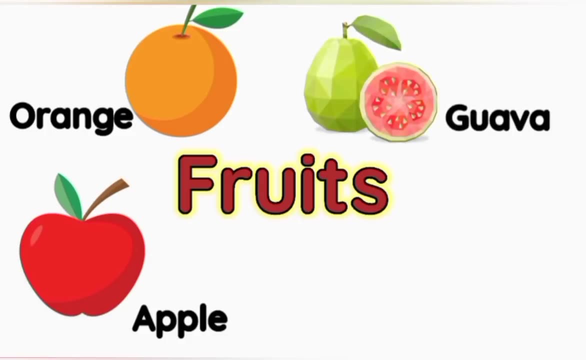 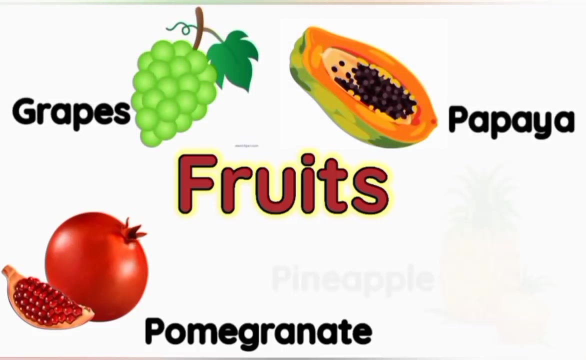 and the nights get longer. Winter season also gives us variety of fruits and vegetables, such as apple, orange, guava, strawberry, pomegranate, grapes, papaya and pineapple. We also get cauliflower, spinach, peas, beans and some vegetables. 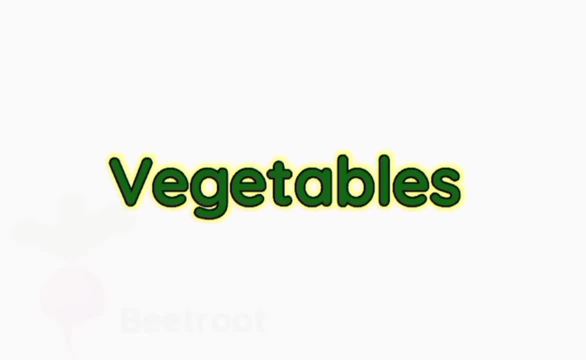 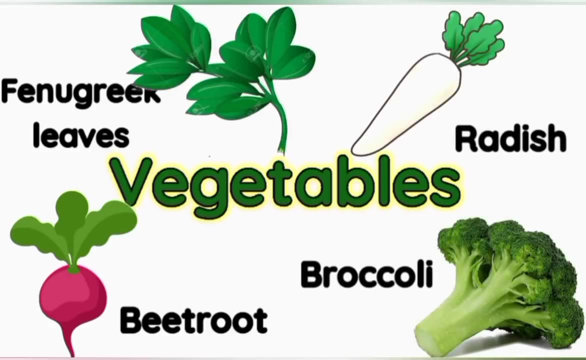 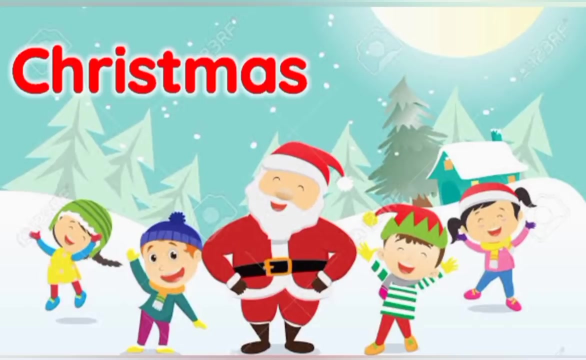 Winter season also gives us variety of fruits and vegetables, such as apple, orange, guava, carrots, beetroot, fenugreek leaves, radish and broccoli. Christmas falls in the winter season. Children wait excitedly for Santa Claus' sleigh expecting. 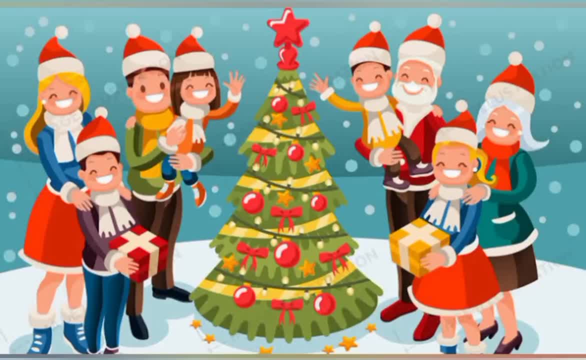 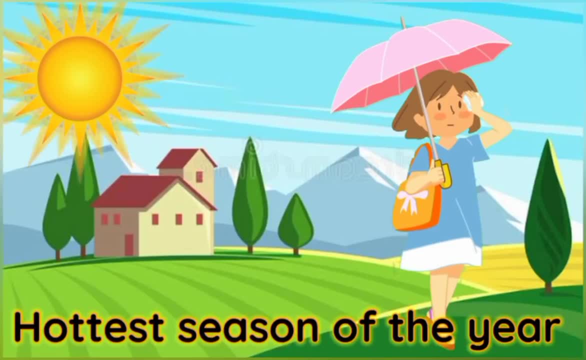 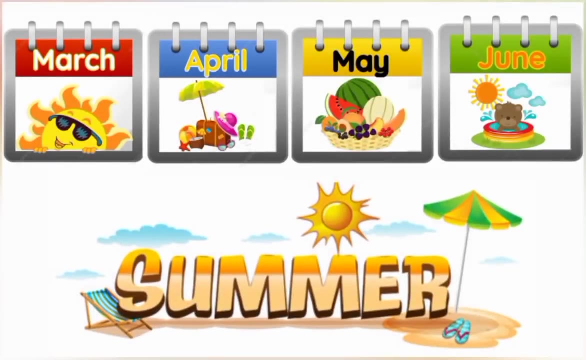 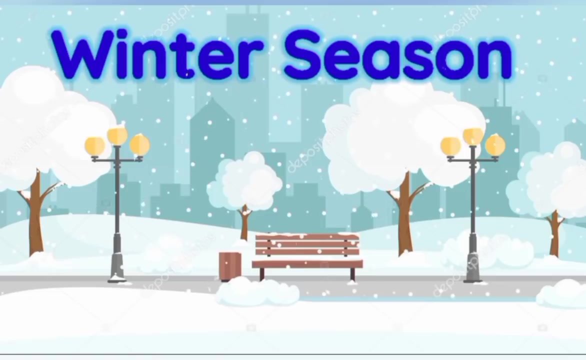 gifts from him. Now we will know about the summer season. Summer is the hottest season of the year, which starts in the month of March after Holi and lasts till June or July. Summer season comes after the winter season. The weather during the season is very hot. 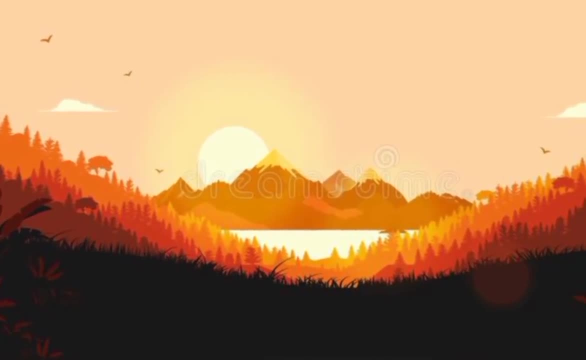 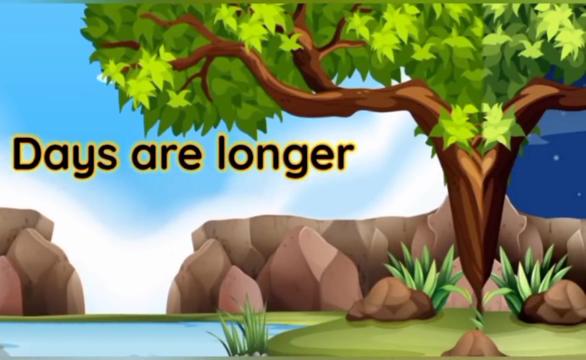 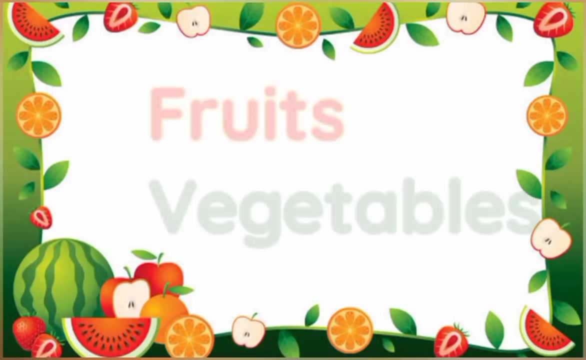 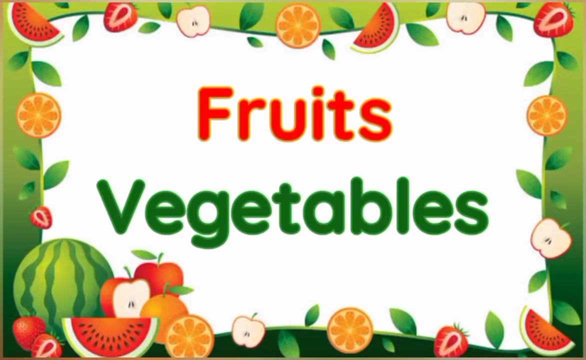 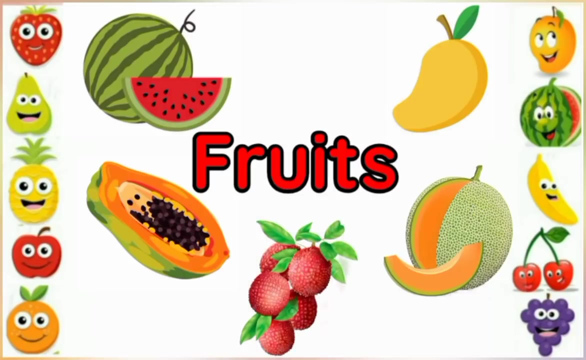 The temperature can stay warm even after the sun has gone down at night. During this time, the days get longer and the nights get shorter. During the summer season, our nature gifts us variety of fruits and vegetables rich in water, such as watermelon, mango, papaya, muskmelon and lychee. 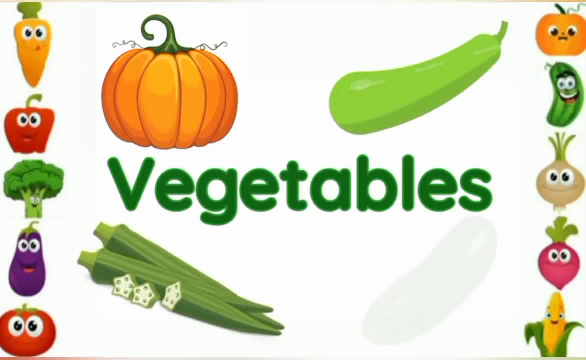 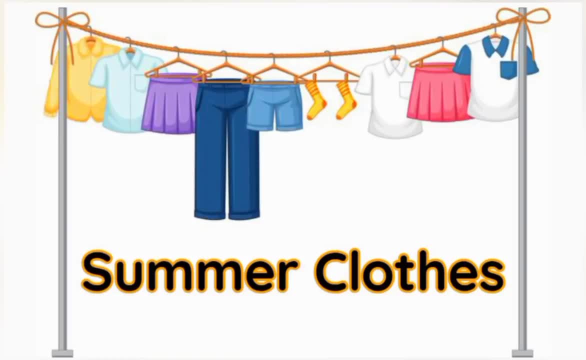 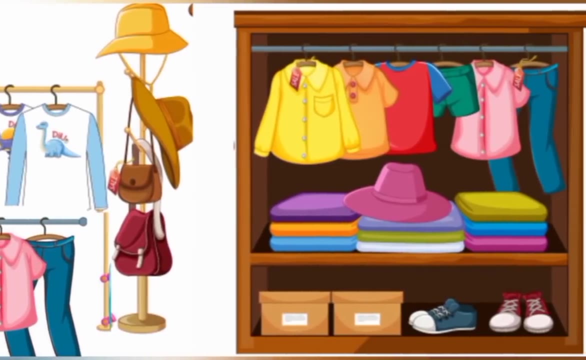 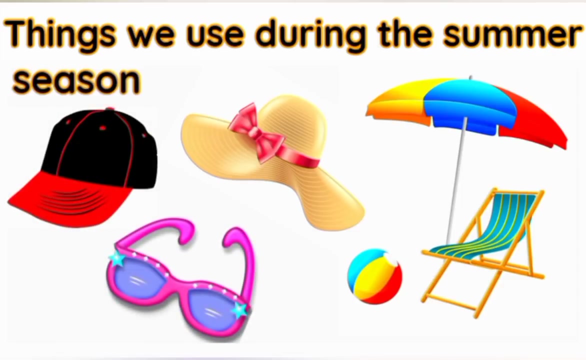 Pumpkin, Pumpkin Bottle, gourd, Lady's finger and cucumber Summer clothes. People prefer to wear light-colored cotton clothes. due to heat, They also use hat, amorella, cap and sunglasses for escaping from sun. We also use air coolers and tassels. 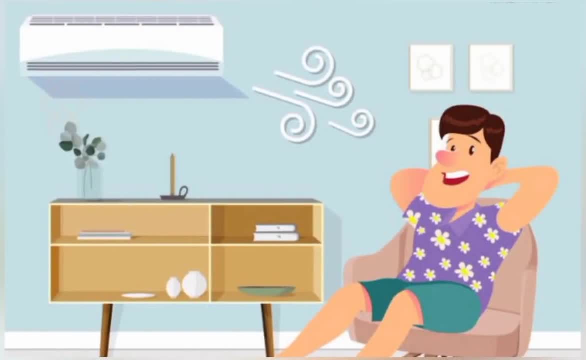 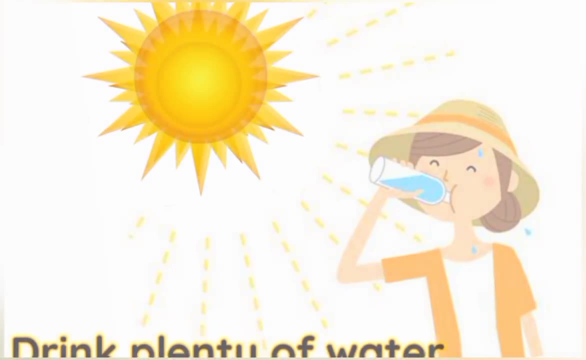 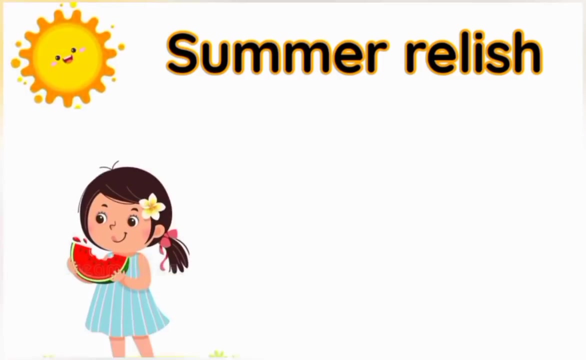 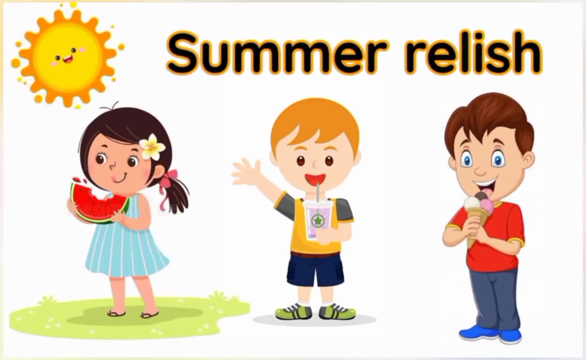 We also use air conditioners to keep our surrounding school During the summer season. we must drink plenty of water to keep ourselves hydrated. During this season, children relish a lot of fresh fruits, juices and ice creams. Summer season is the most entertaining season for kids. 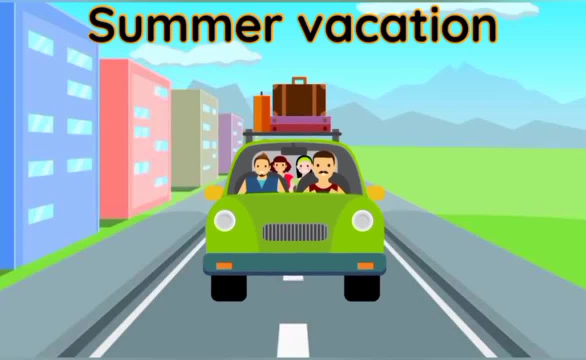 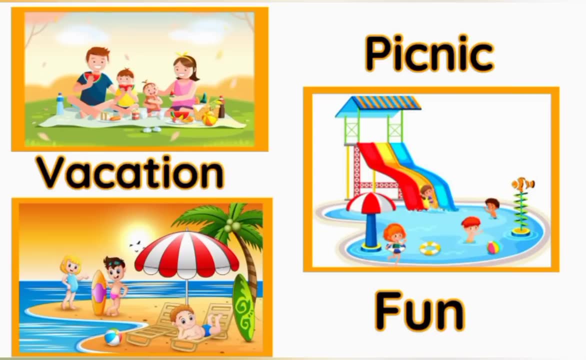 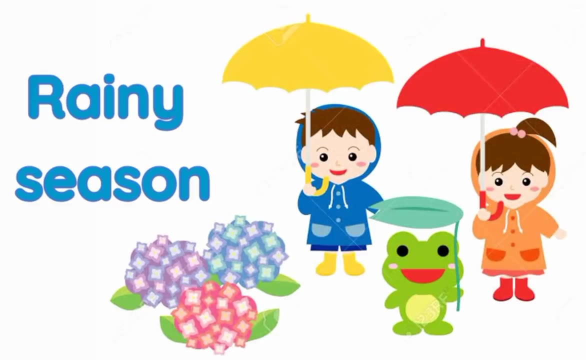 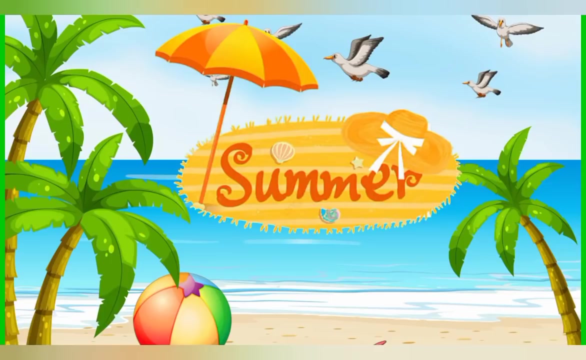 As it's the time when the school gets closed and the vacation begin. For children, summer season is the time of vacation, picnic and fun. Now we will know about our rainy season. Rainy season comes after the summer season, which starts in the month of June and extends. 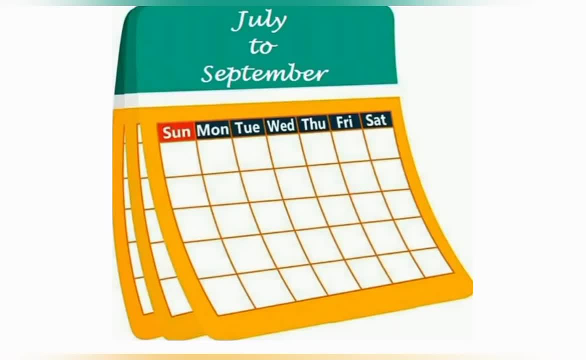 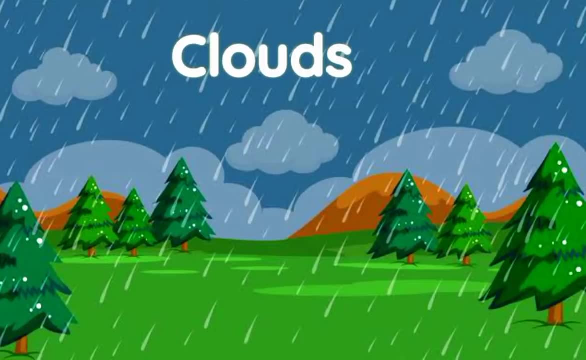 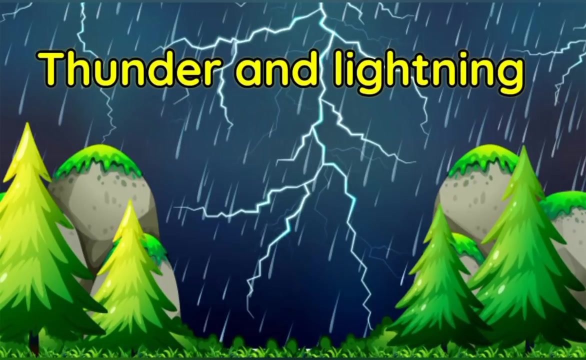 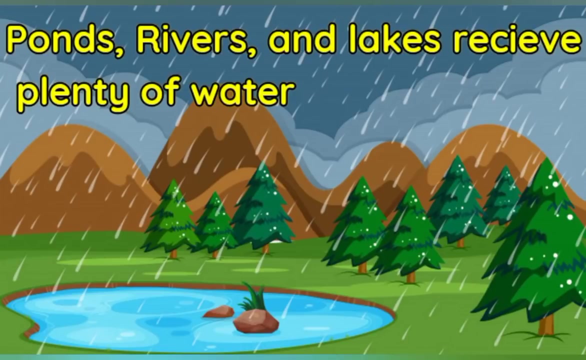 up to September. We also call it as monsoon season. During this time, the sky looks cloudy, with heavy black clouds. Everywhere, there are sounds of lightning, with huge, tremendous thunder. We often see rainbow as well. Ponds, rivers, streams, Rivers and lakes receive plenty of water during the rainy season. 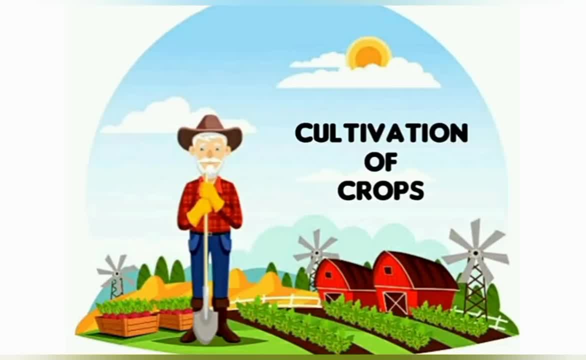 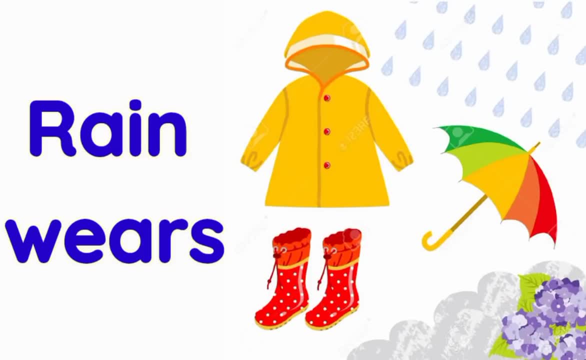 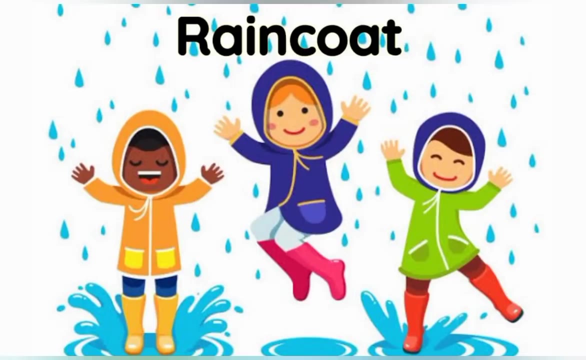 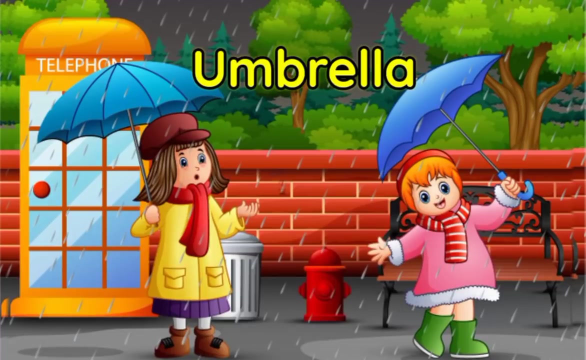 It also helps farmers, as they get plenty amount of water for good cultivation of crops. In order to protect ourselves from rain water, we use rain wears such as rain coat, umbrella, rain shoes, rain mask and gum boots. We also get variety of fruits during the rainy season, such as peaches, plum, leechi and cherries.